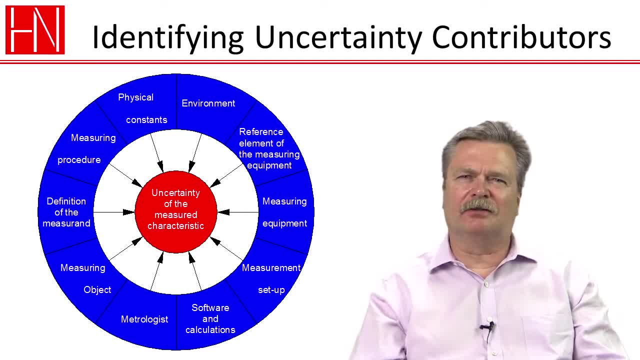 how. that, in a sense, is the most important part of the uncertainty estimation process, because if we don't find the significant contributors And, as I kept saying, telling you, as long as you can find the three major contributors, your budget is going to be as good as it can be. 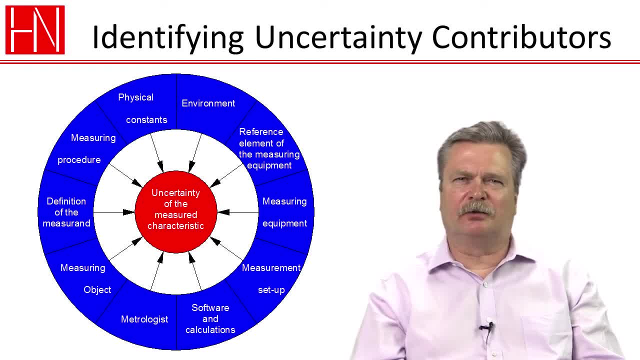 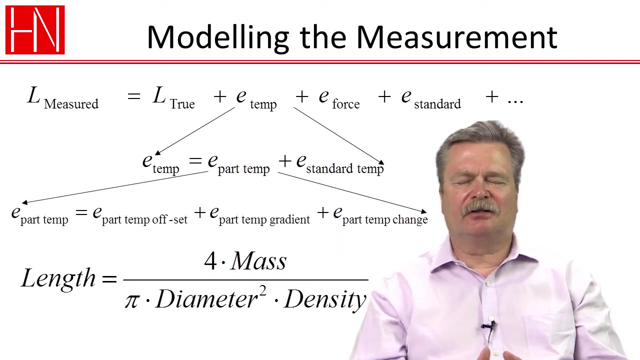 But if you cannot successfully identify the three largest contributors, then all bets are really off on whether your uncertainty- the uncertainty that you calculate- is anywhere in the vicinity of what the true uncertainty of your measuring process is. Then, once we had identified the uncertainty contributors, we started talking about how to model the measurement. 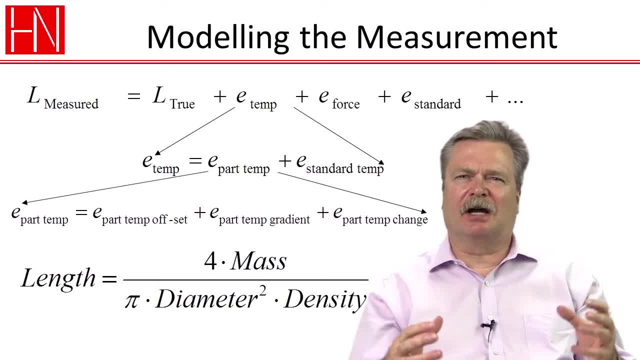 And by modeling the measurement. I'm talking about how the uncertainty contributors and the measured value, what we call the measure-and- are linked together, And we talked about how that is sometimes more of an art than a science to decide how much detail to really focus in on or zoom in on, and where you limit that to. 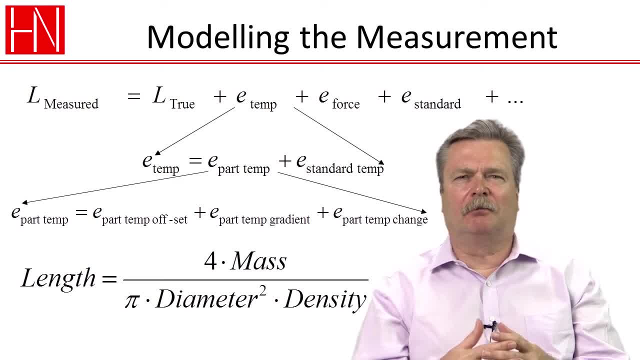 So you don't make the job too complex and impossible for yourself. We also talked about the idea of there sometimes being more complex kinds of equations and went through the example of trying to determine the length of a cylinder by measuring the mass, the diameter and the density of it, and how we then take the base measurements. 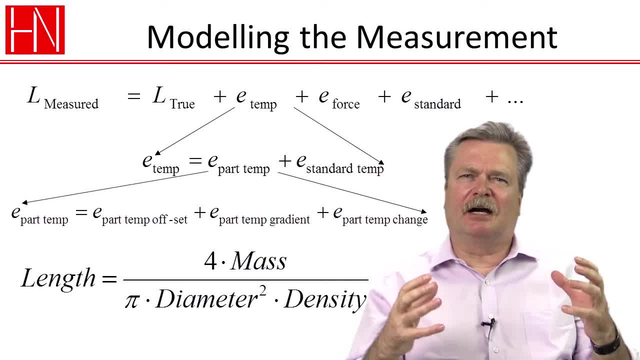 those three individual measurements and the uncertainties of them and how we then combine them together for an overall Uncertainty of the length determination. Then we talked about the core of it, which is the GUM method and I'm sure you know by 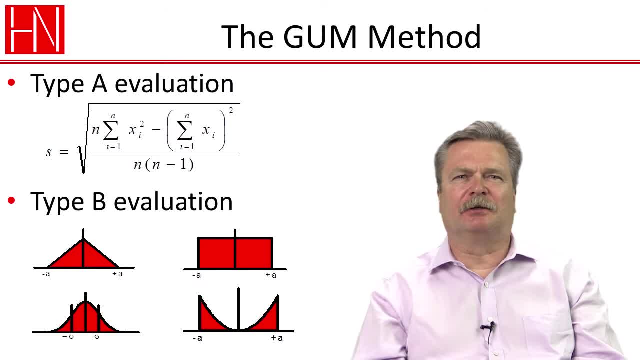 now that GUM stands for the Guide to Expression of Uncertainty in Measurement, and how that is fundamentally built on the idea that there are two different ways of evaluating uncertainty contributors: one that we called, or that GUM calls, a Type A evaluation, where you calculate. 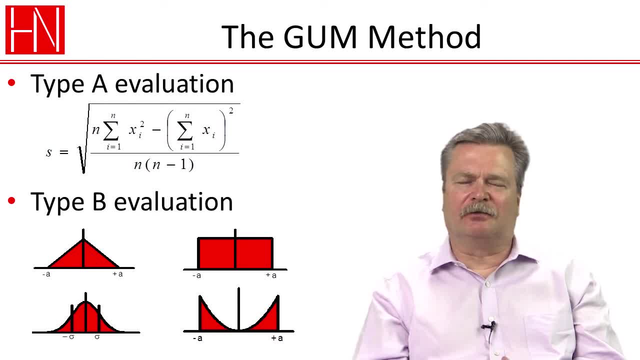 the standard deviation directly from repeated observation. That is, you make a number of measurements and then you calculate the standard deviation, typically through a spreadsheet. And then the other way of estimating uncertainty contributors, and the one that probably was the most revolutionary when the GUM method was first put forward, was the Type B evaluation. 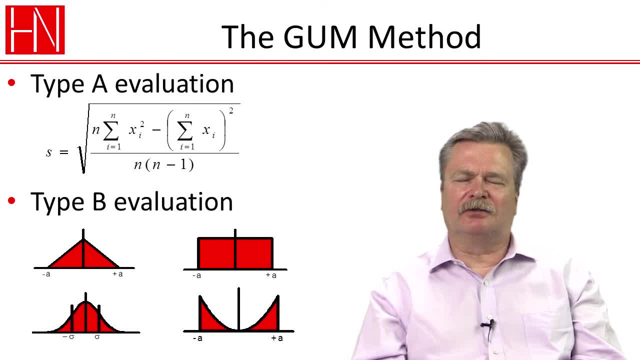 where the way we evaluate the uncertainty contributor And then the other way of estimating uncertainty contributors is that we come up with a set of variation limits, either from prior knowledge or from manufacturer specifications, or from information in a calibration certificate or any other information that's available. 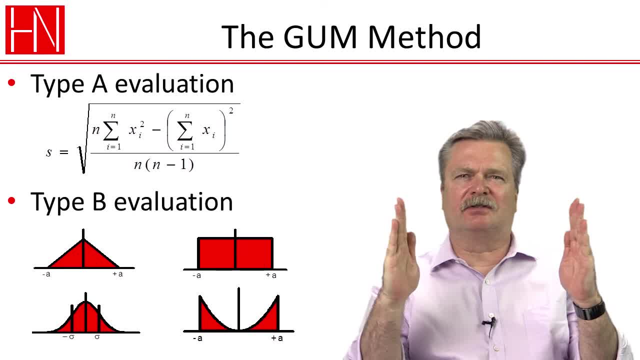 to us. we can come up with a set of limits and say, well, this influence stays within these limits. And then we talked about how we can then assume a distribution between those limits, and we talked about which distributions are Appropriate in which cases. 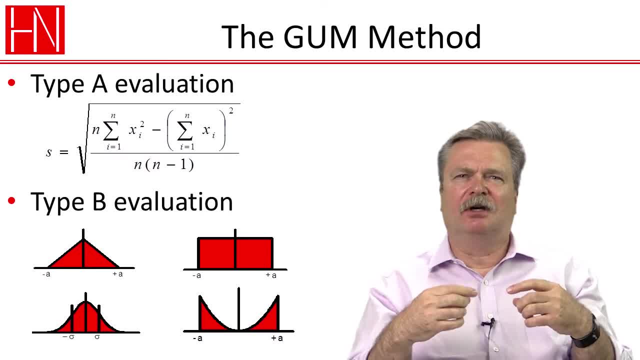 And from that we can calculate an equivalent standard deviation. so we could get all of our contributors into a format where each of them has the weight of one standard deviation and that standard deviation is calculated in terms of how much it influences the measure and the value that comes out of our measurement. 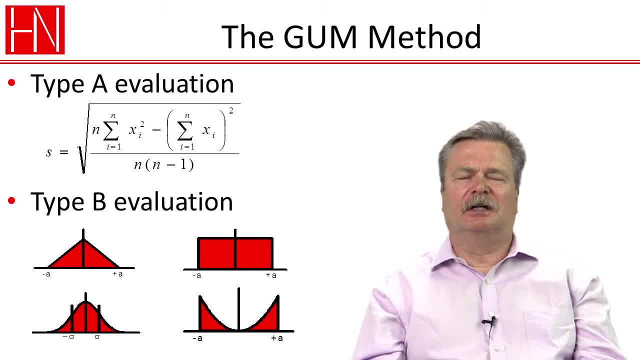 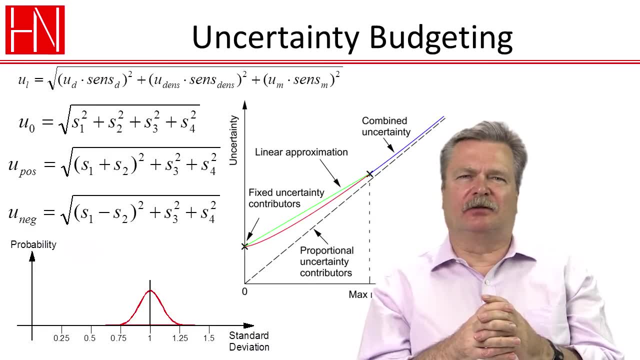 And that was what we needed to do to be able to add them together. Then we talked about how we then add these contributors together, and we talked about how to add uncorrelated contributors together as the square root of sum of squares, And we talked about, if we have correlated contributors, how we would add those linearly. 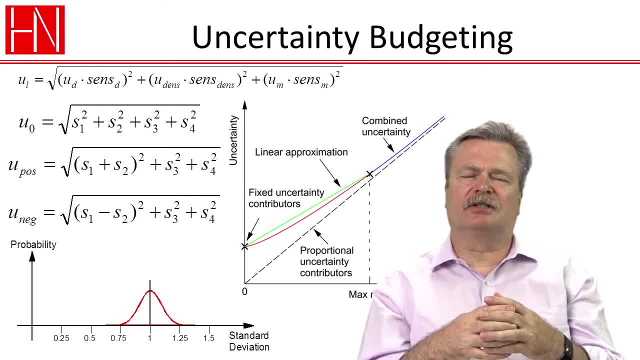 or subtract them from each other linearly, depending on whether it's positive or negative correlation, before we square them together with the remaining contributors. We also went through the details- Details of when we have a complex measurement situation like the one where we determined. 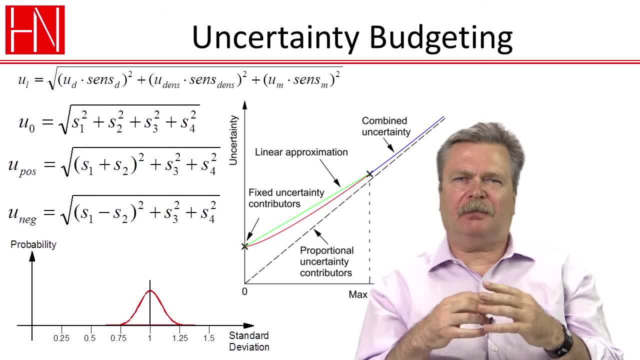 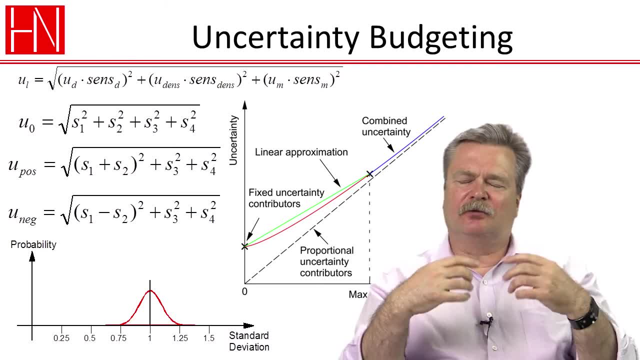 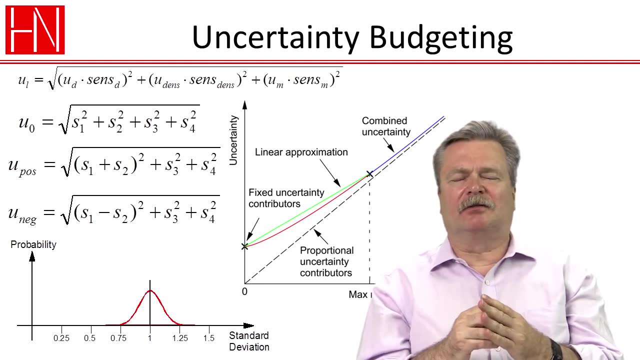 the length, from the diameter, the density and the mass, how we then have to calculate a sensitivity coefficient for each of the measurements to find the overall uncertainty for the entire measurement. We talked some about the limitations of our uncertainty estimation, The limitation of the 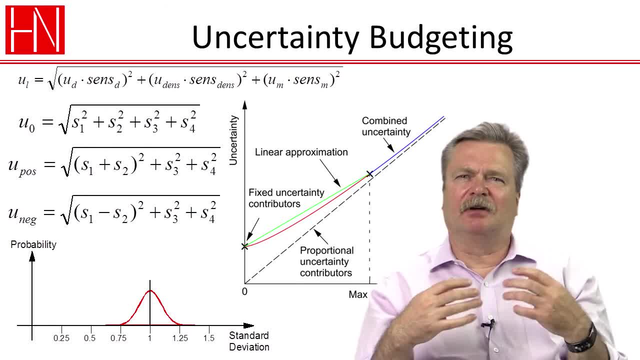 The knowledge we have of a standard deviation when we have a limited number of samples, And I emphasized that really you should have at least 30 measurements for every time that you calculate a standard deviation, Otherwise really the uncertainty of that standard deviation is unacceptably high. 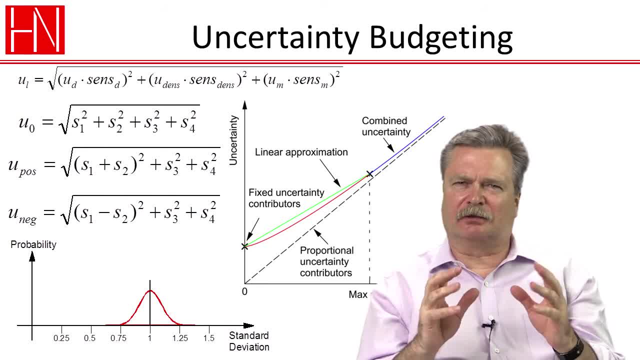 There are some tools that you can use to sort of correct for it, but mathematically that's quite complicated And we didn't really get into that in any detail In this course. What we did talk about was that sometimes you have a measuring process where it's the 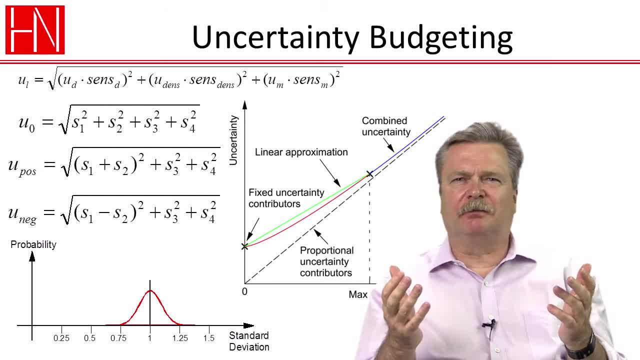 same over a range for typically for a particular measuring instrument And we talked about how we can make a linear statement out of that, because for the vast majority of measuring processes there will be some fixed uncertainty contributors and some uncertainty contributors that are depending on the measured values. 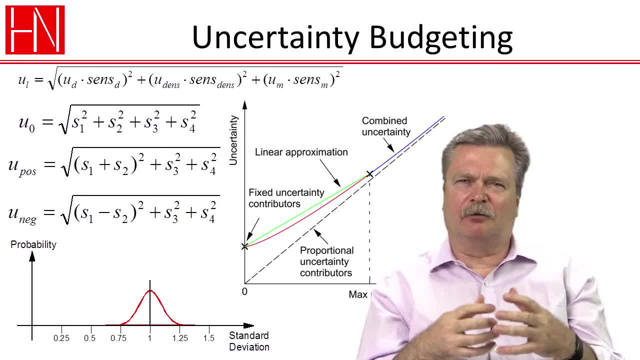 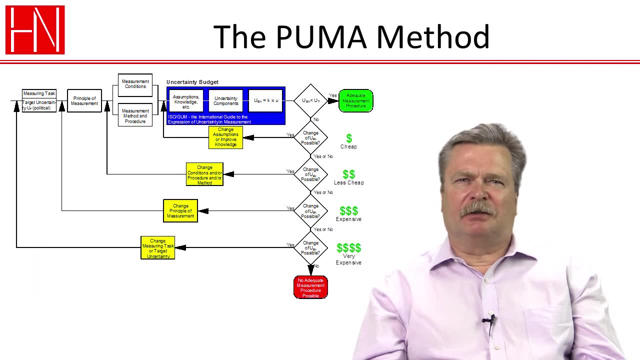 And so we talked about how we can make a linear expression out of that that can make a simple and convenient way of expressing the uncertainty of that process over the given range. And then, finally, we talked about the PUMA method, which is this iterative way of doing. 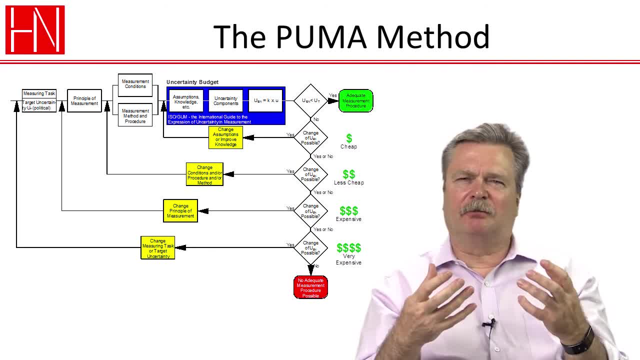 uncertainty budgeting, where we first come up with some initial estimates that are, you know, As far as possible type B evaluation and as simple and as quick as possible, And where the idea is that, rather than find that elusive true uncertainty, we say what? 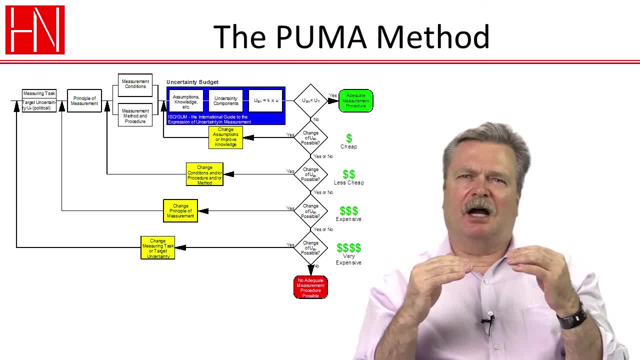 we want to do is to make sure that our uncertainty is less than some target value. Maybe we're measuring parts and we want the uncertainty to be less than 10% of the tolerance, So we have a four to one ratio. We want to keep between the uncertainty and the specification for an instrument we're calibrating. 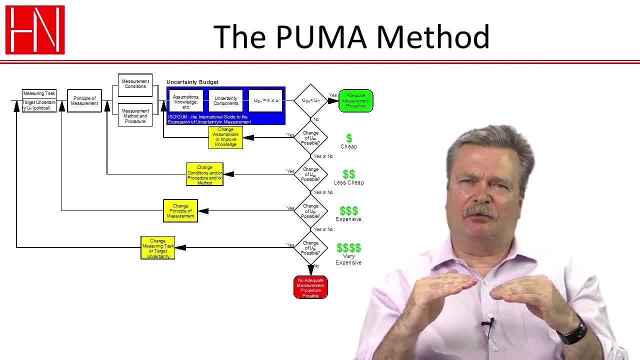 for example. And so the idea is that we say we estimate on the high side. So we say, well, we don't know what this contributor is, but we're pretty sure it's not more than this. And if, when we evaluate that way and we're still less than the target uncertainty, then 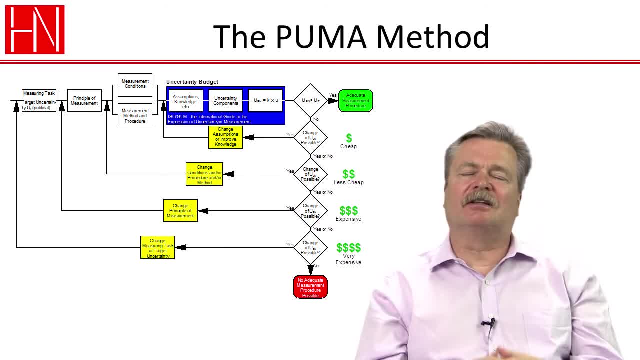 we know that that true uncertainty is also less than the target, And that's what we do with the PUMA method. And then, finally, we talked about the Puma method. We talked about how we can use that PUMA method in sort of a predictive way of estimating.